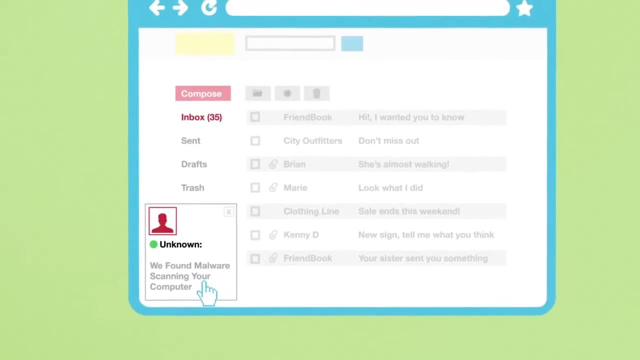 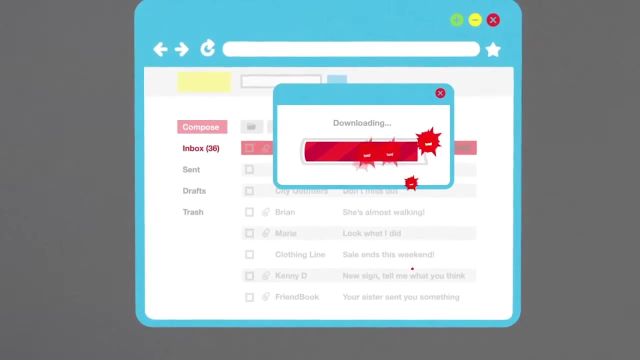 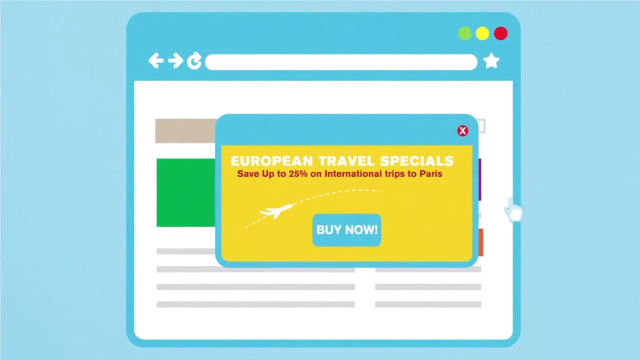 if they say they scanned your computer and found malware. Scammers send messages like these To trick you into buying worthless software or, worse, downloading malware. what else can you do? Use a pop-up blocker and don't click on links in pop-ups. Don't click on links. 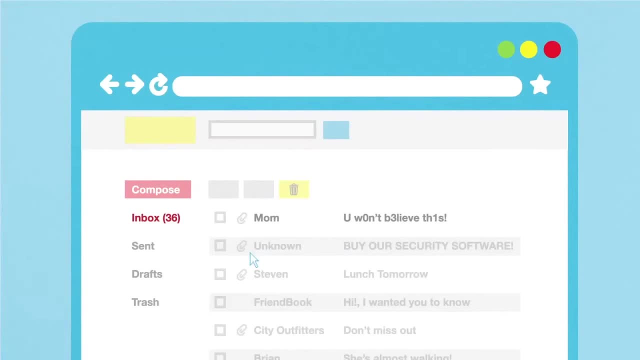 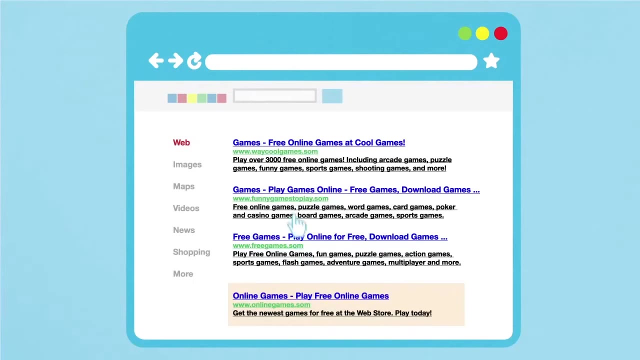 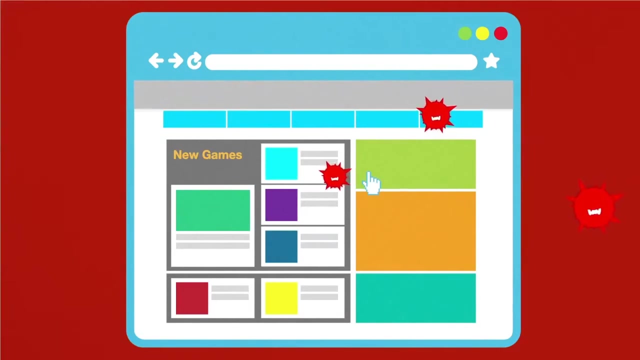 or open attachments in emails unless you know what they are, even if the emails seem to be from friends or family. Download software only from websites you know and trust. Free stuff may sound appealing, but free downloads can hide malware. Make sure your web browser's security setting is high enough to detect unauthorized downloads. 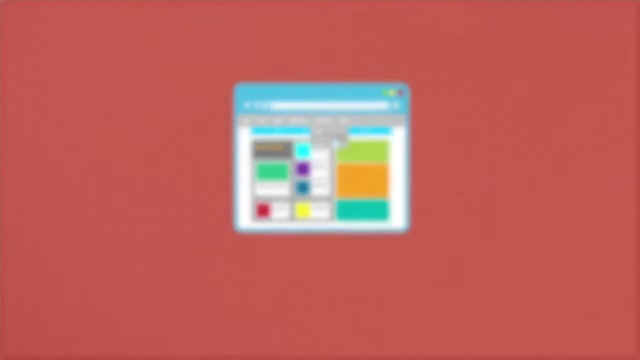 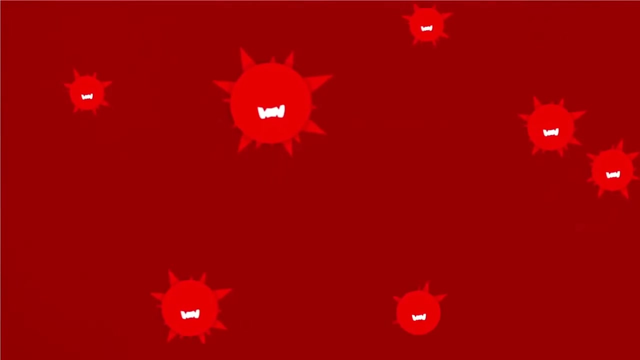 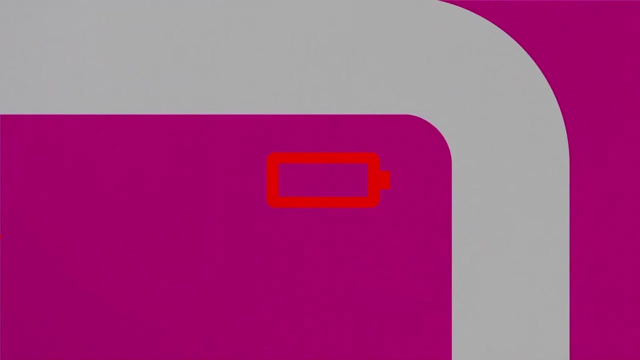 For example, use at least the medium security setting. Even if you take precautions, malware can find its way onto your computer. So be on the lookout for these signs: Your computer runs slowly, drains its battery, quickly displays unexpected errors or crashes. If your computer 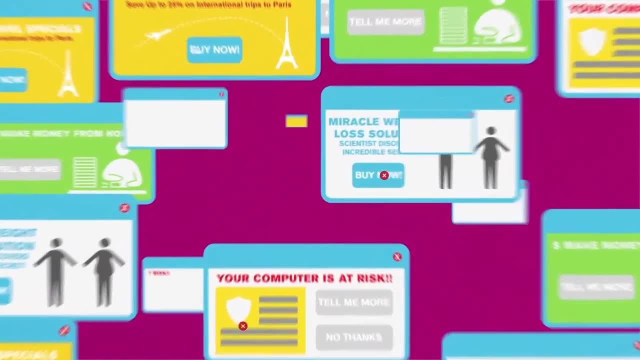 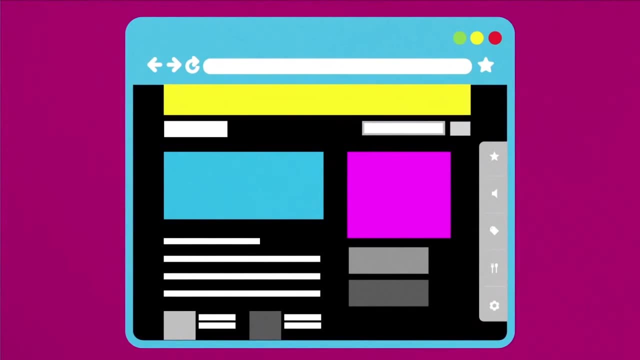 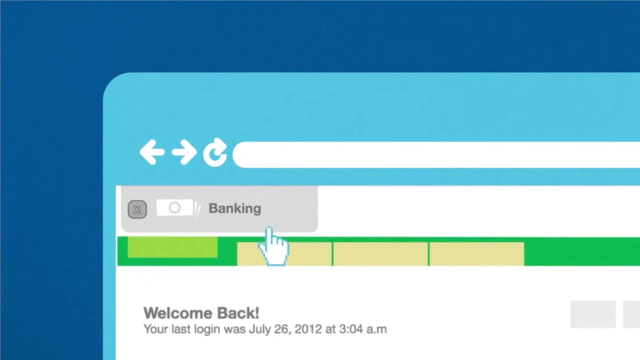 won't shut down or restart. it serves a lot of pop-ups, takes you to web pages you didn't visit, changes your homepage or creates new icons or toolbars without your permission. If you suspect malware, stop doing things that require passwords or personal info, such 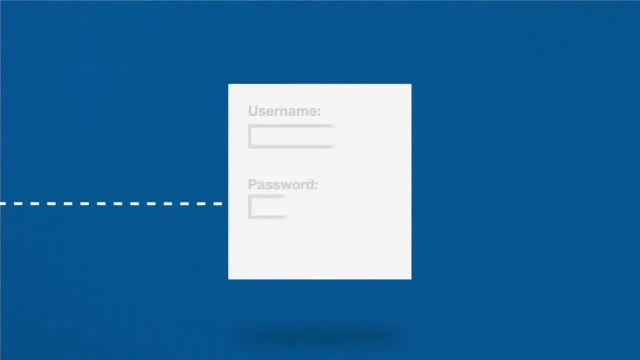 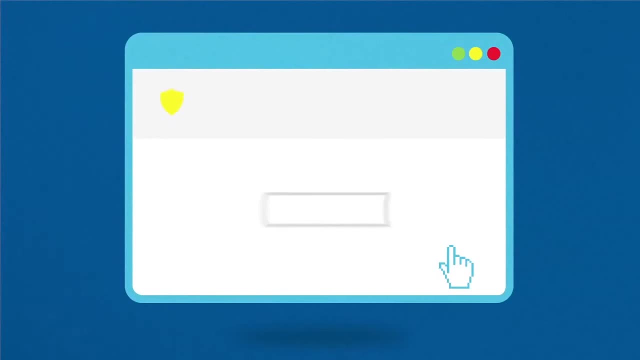 as online shopping or banking. Use a different computer, maybe one at work or at your local library, to change your passwords, Update your security software and run a system scan. Delete files it flags as malware. If you can't fix the problem on your own, get help from a professional. Your computer. 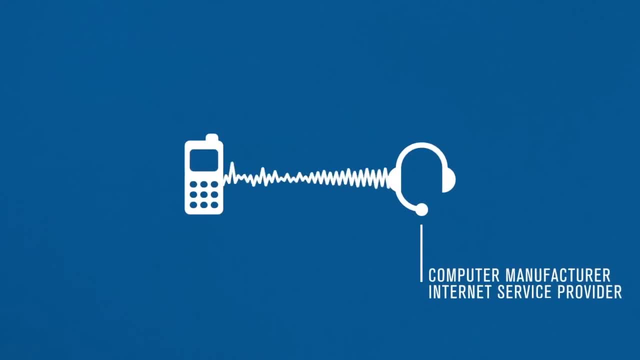 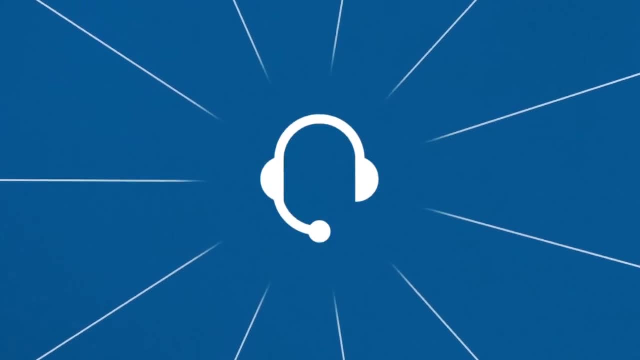 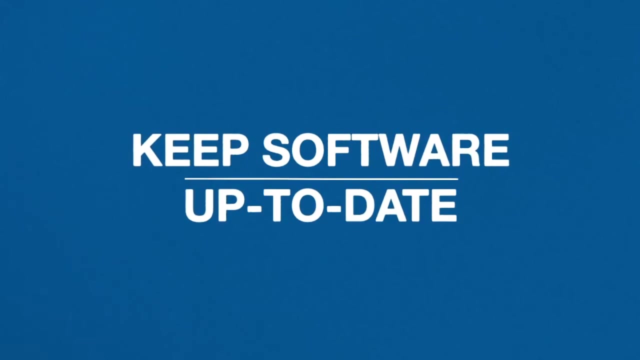 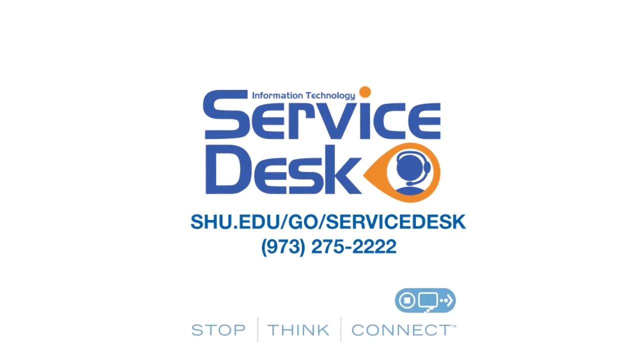 manufacturer or internet service provider may offer free tech support. If not, contact a company or retail store that provides tech support. Keep in mind the most important thing you can do to prevent malware is to keep your computer's software up to date. If you're having trouble with malware or viruses, contact the Seton Hall University. 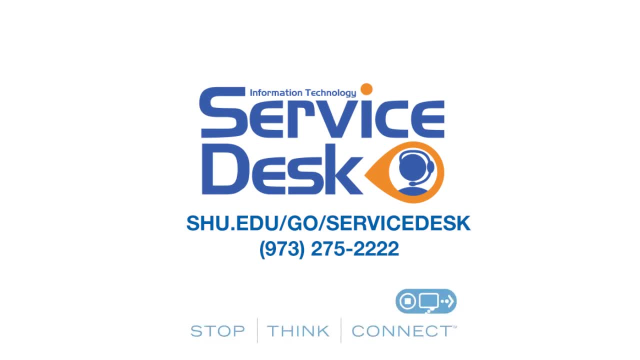 Service Desk at shuedu slash go slash servicedesk or 973-275-2222..